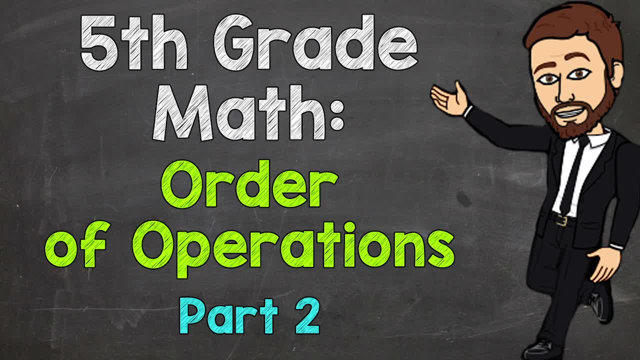 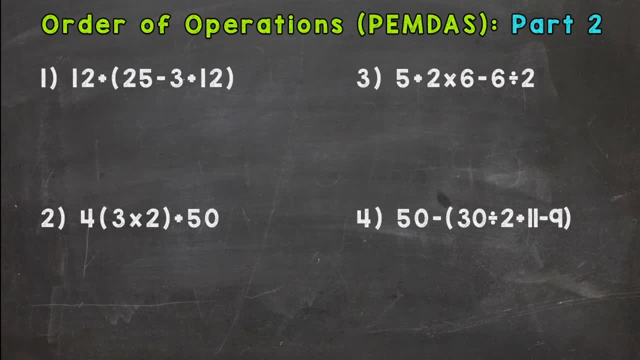 Here we have order of operations, part two, where we are going to do four problems that build upon the problems we did in part one. These are a little bit harder and more complex, a little bit longer too, to solve more steps. So if you're looking for part one and you missed part one, 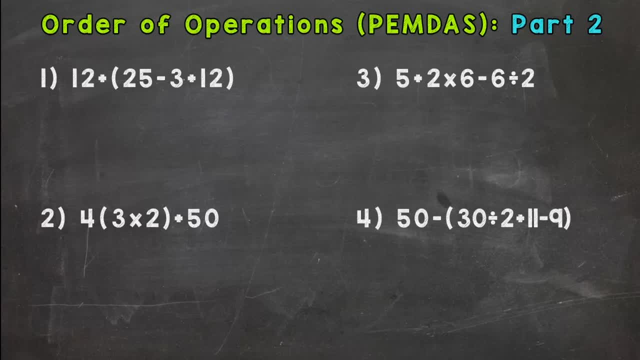 I dropped the link down in the description. I highly suggest you check that out before part two. Part one has more of an introduction about the steps we use to solve these problems. If you're ready for part two, we're going to start here in a second. Remember you don't solve these problems. 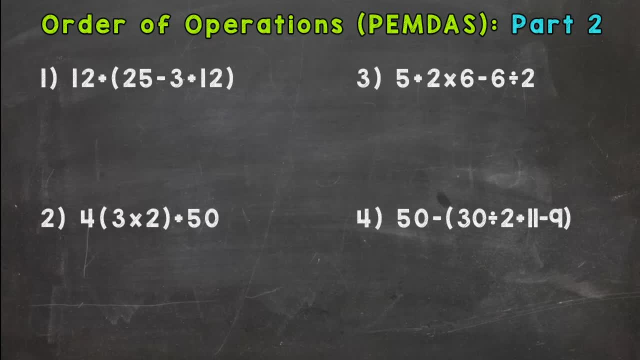 in any order you want and you don't go from left to right. You use that certain set of instructions or steps and you remember them with the acronym PEMDAS. I gave you a little table that looked like blocks stacked up. It was on the left hand side of your screen, in part one. I suggest you 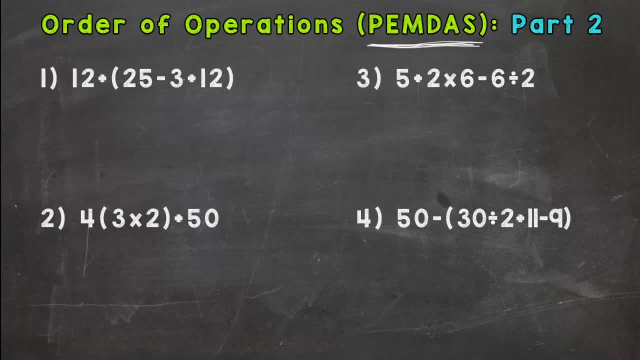 copy that table down and use that as you go through these problems until you have the steps memorized. So for part two, I would highly suggest you write these out with me. That will be better for you as far as learning the process of how to do this, And then we'll follow up part two. 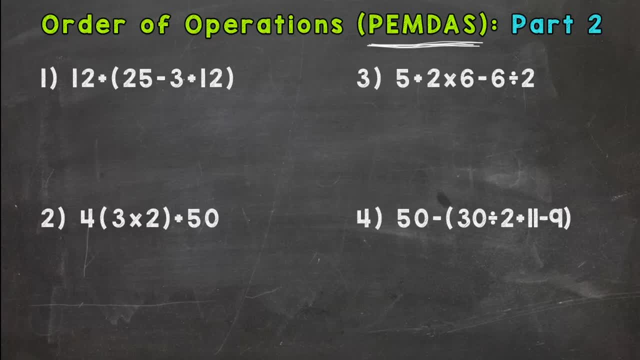 this video with the mastery check which I dropped, that link in the description where you will try some on your own to see if you're good to go with order of operations problems. So let's start with number one here, And we have 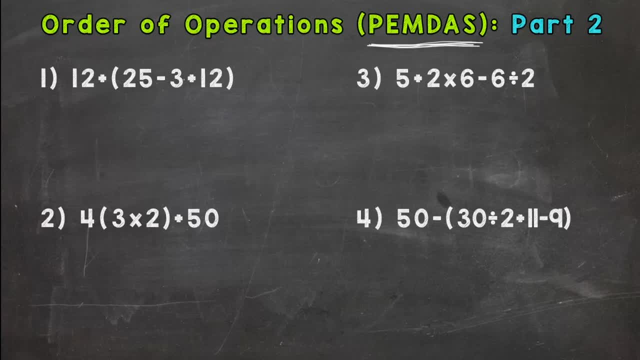 addition, parentheses: subtraction and addition. So our first step is always anything in parentheses. So we're going to take a look at the 25 minus 3 plus 12.. So our options are subtraction or addition. first, Addition and subtraction are both priority for or at the bottom of our order of. 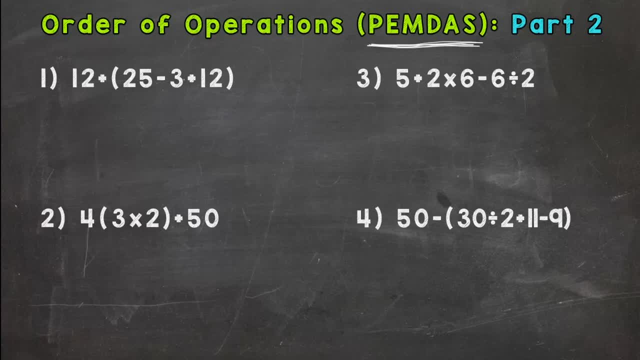 operations. So we go left to right because addition and subtraction kind of hold the same weight. They're both on the same level. So we do subtraction first. 25 minus 3 is 22.. Bring down everything we didn't use. And we still bring down the parentheses. 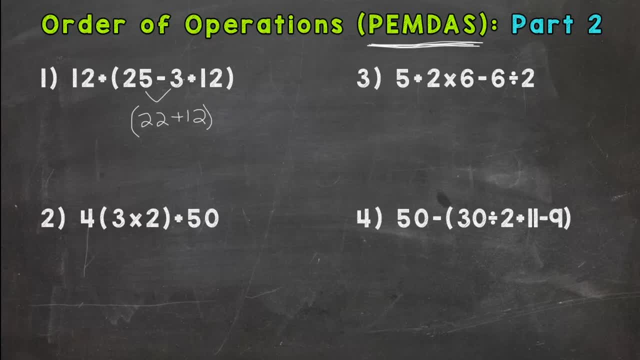 You only get rid of the parentheses when you use up every operation inside of those parentheses. That's when they will go away. And don't remember to drop, or don't forget to drop your 12 and addition sign. So let's look at this line now: We have 12 plus parentheses, 22 plus 12, and parentheses. So let's. 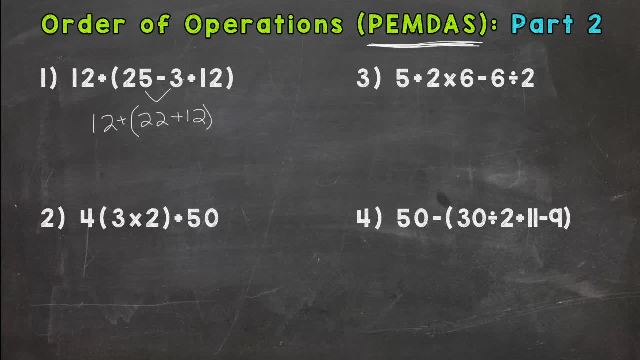 go through our steps. Do we have any parentheses? Yes, So automatically start with that: 22 plus 12, is 34.. Now we used up all of the operations within those parentheses, so they go away. Drop your addition sign and your 12.. And now we only have one thing left. So obviously, that's what. 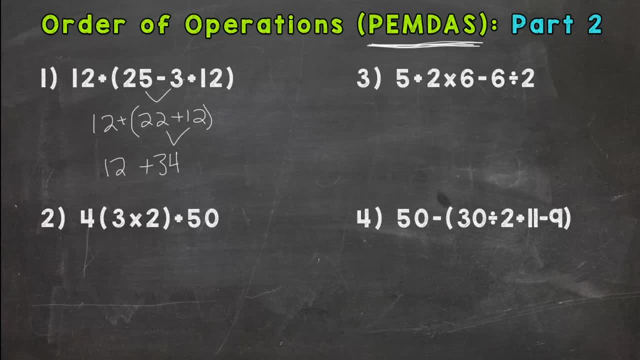 we do 12 plus 34, and I'm running out of room, So I'm just going to put an equal sign here And that gives us 46. Circle, your final answer. There we go. We showed all our work. We showed all our steps. We were careful about how we solved the. 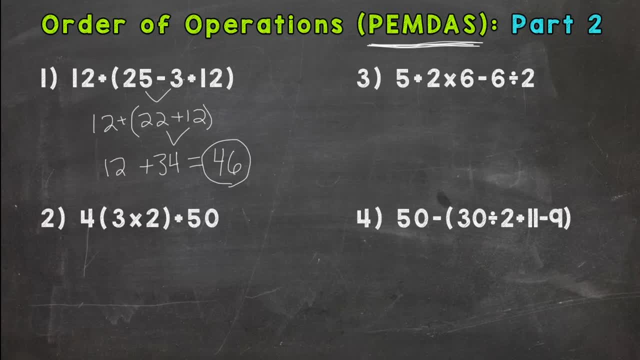 problem Forty-six. We are good to go. Number two: We have a 4 right up next, right up next to the parentheses. so hopefully we remember what that means: A three times 2 in the parentheses And then a plus 50.. So let's go through our. 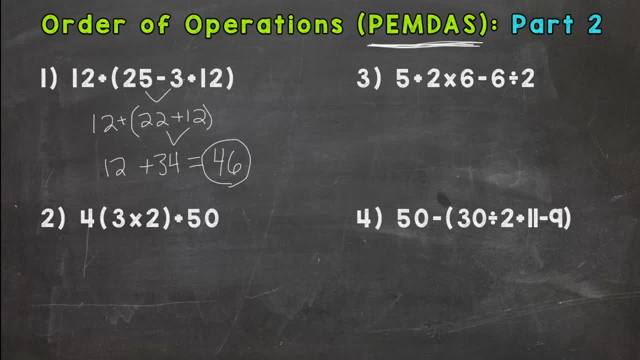 steps. Any parentheses? Yes, So we start there 3 times a 6. We used all of the operations in those parentheses, so they go away. now Let's drop the 4.. And what do you think comes between the 4 and the 6?? Hopefully you're thinking. 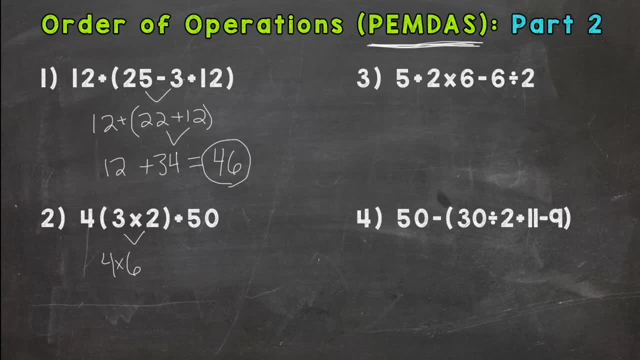 multiplication. Whenever a number is right next to parentheses, it means multiplication. You can even put an x in here in the original problem if you don't like having the number right next to the parentheses. It means the same thing. And then drop our plus 50.. Let's. 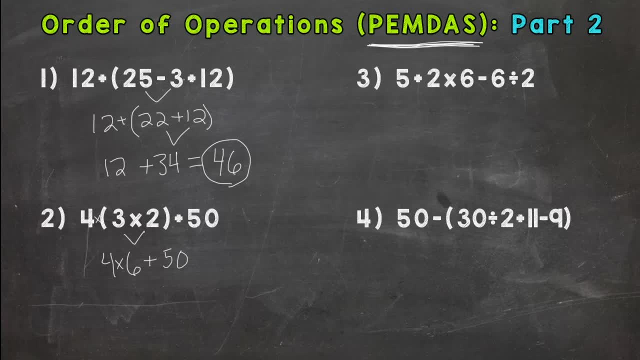 go through our steps. Any parentheses now No, Any exponents, No Multiplication or division. Yes, We have multiplication 4 times 6. Hopefully you're thinking 24.. And then plus 50. And 24 plus 50, we get 74.. 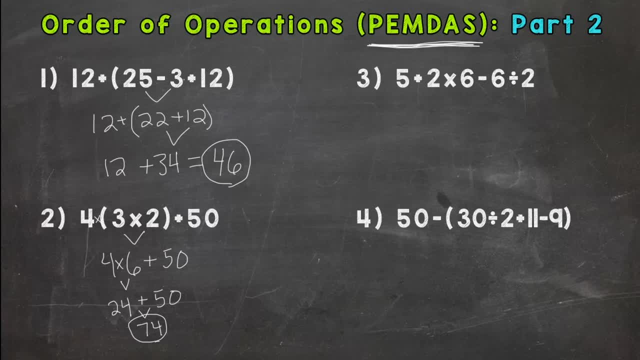 We showed all our work, We took our time, We went through our steps. Good to go with number 2.. All right, Number 3 is a little bit different than all of the problems we've done so far because there aren't any parentheses. So let's go through our steps. Any parentheses? 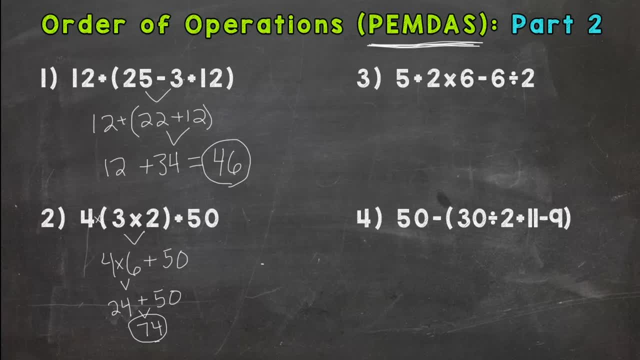 Well, we just said no, So we need to go to e exponents, Any exponents, No Multiplication or division. Yes, We have both. We have multiplication and division, So they are both level 3. And they're both the third priority. So that means we go left. 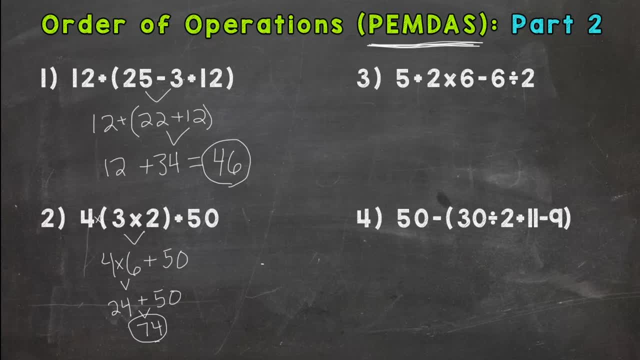 to right. We do whatever comes first And that's multiplication. So 2 times 6 is 12.. Now we need to drop everything we did not use. Oops, That should be 6 divided by 2.. Let me put a division sign there. All right, So we have addition, subtraction and division. 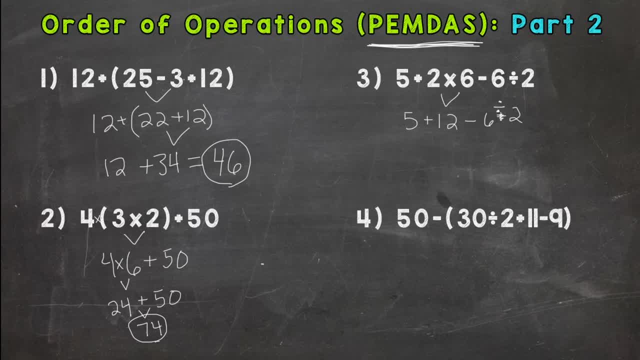 Any parentheses, No Exponents, No Multiplication or division. Yes, So the 6 divided by 2 will give us 3. Drop everything we did not use. All right, We have addition and we have subtraction, So those are both level 4. Right: Addition, subtraction are both the fourth instructions. 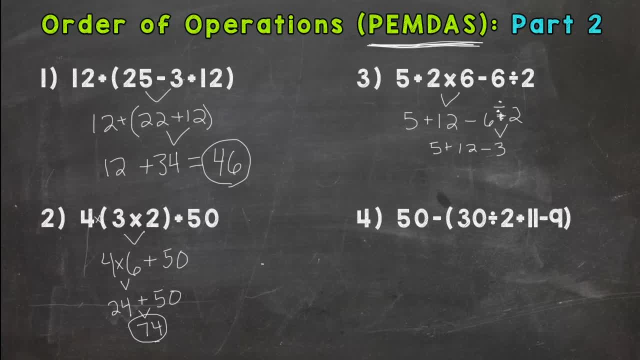 or steps down that set of instructions. we use Left to right Whatever comes first: 5 plus 12,, 17.. And drop our minus 3.. 17 minus 3, I'll put an equal sign is 14.. Done Okay. Now notice on 1 and 3,. on my final step, I 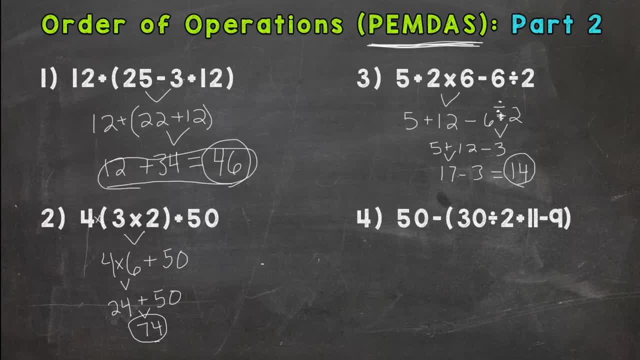 put 12 plus 34 is 46 equals 46. Or 12 plus 34 equals 46. That's fine. Or number 3, I'm putting: 17 minus 3 equals 14. And then number 2, I continue down with that arrow or partial. 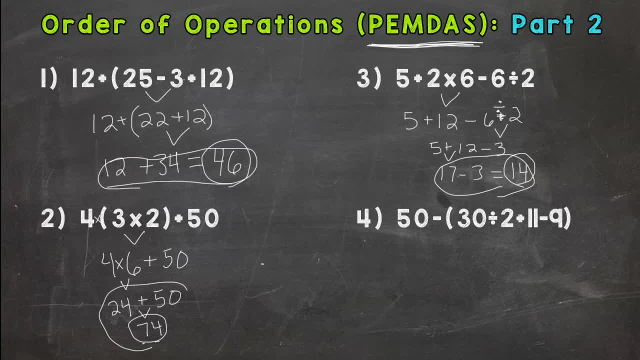 triangle method and circle the 74 under that final step. Any way, any of those is fine, The equal sign or just continuing down, It doesn't really matter, as long as you get to the correct answer, Number 4.. Any parentheses: Yes, And we have 4.. All right, Let's go ahead.